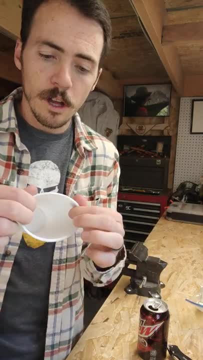 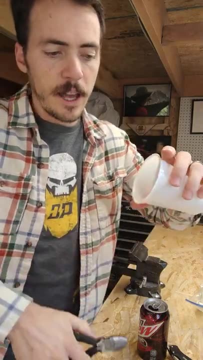 so there might be some irreversible damage happening here, but overall these are much tougher. They're much tougher to break right. In fact, I can take these and even if I cut it right, if I apply an additional flaw where this thing has been cut, all of a sudden it becomes. 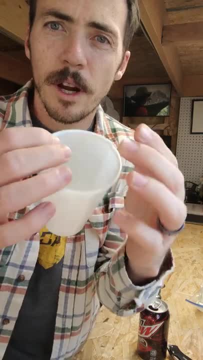 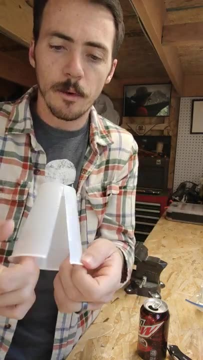 much easier to fracture, where, if I tried that without the flaw, it doesn't break at all. So something about having an initial flaw and then having an additional flaw and then having an initial flaw makes it easy for that thing to break into two pieces, right? And if we continue, 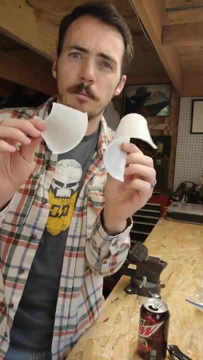 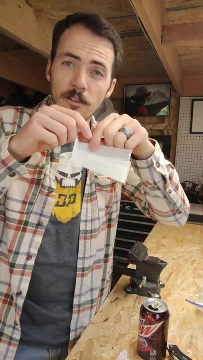 this would probably continue all the way until we have two separate components, and that's when you have fracture, right. So this is two pieces. It was controllable. I could keep on applying force and if I applied force, the flaw continued to progress, but that was not the case with the 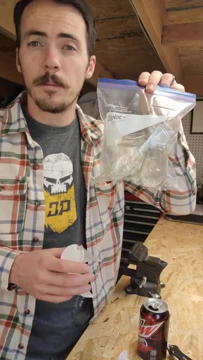 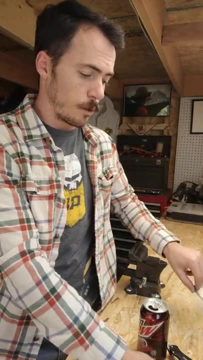 glass, ceramic. Once the flaw started, it continued to propagate in a spontaneous manner. right, I didn't have to keep applying force, It just broke on its own, whereas this thing I had to keep applying force. And what about metals? right, If you take this can, it is also. 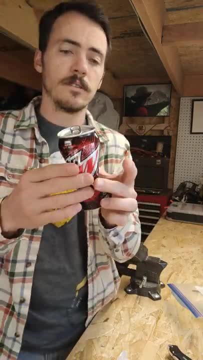 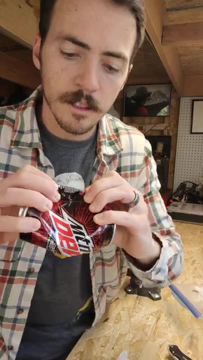 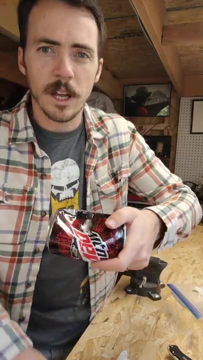 deformable, right, You can deform it and it hasn't fractured into two pieces. and similarly, if I cut this thing, if I apply a cut to it now, you'll see that it's relatively easy to continue that fracture. Let me get it started a little bit better, right? Once we get it going, it's. 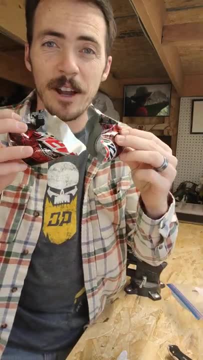 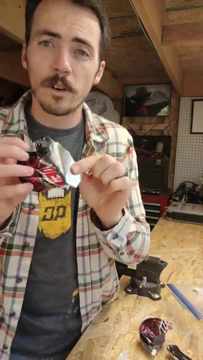 relatively easy to rip it right in half right. Some characteristics of metal and polymers they share is that if you keep on flexing this, we find that over time it would get weaker and weaker and weaker until it would break right. So there's something about. 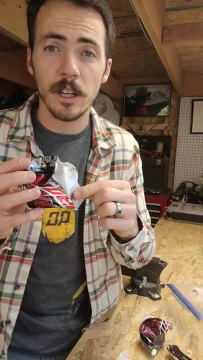 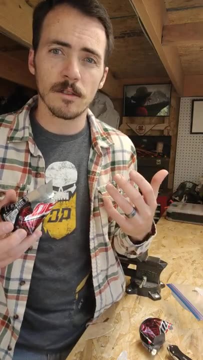 the cyclic nature, where it doesn't break on the first 10,, 20,, 100, even 1,000 deformations, but it might break after 10,000 or a million times. So what's happening to the internal microstructure is something else we're going to cover in this chapter. okay, So that's just a 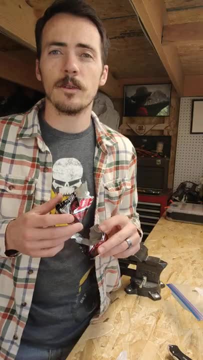 quick primer on the different types of fracture that we're going to see in materials. Now we're going to look at the different types of fracture that we're going to see in materials, So let's.